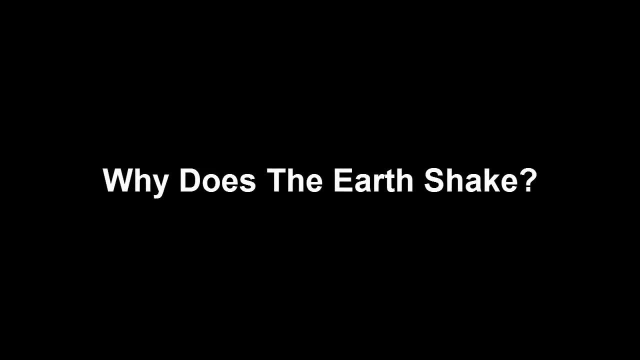 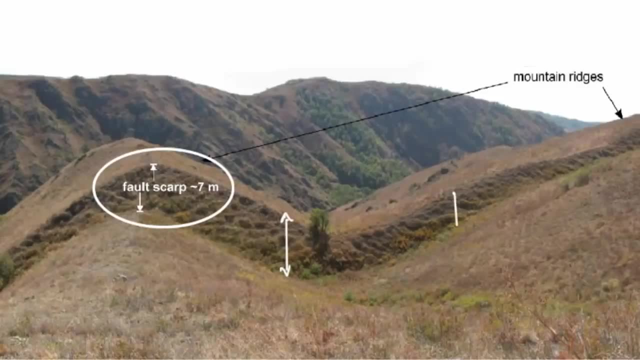 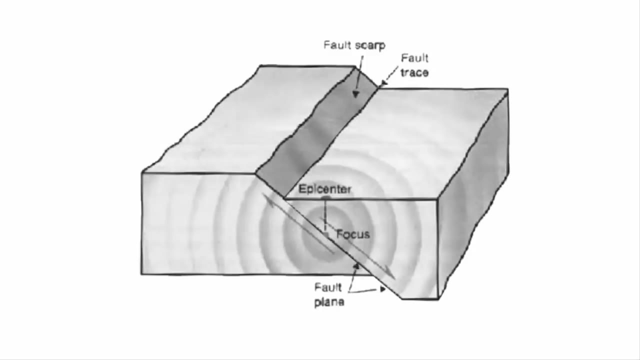 that travel in all directions. Now the question is: why does the earth shake? To understand that, you will have to look at this picture. This is a fault. A fault is a sharp break in the crustal rocks. Rocks near a fault tend to move in opposite directions. That creates friction. 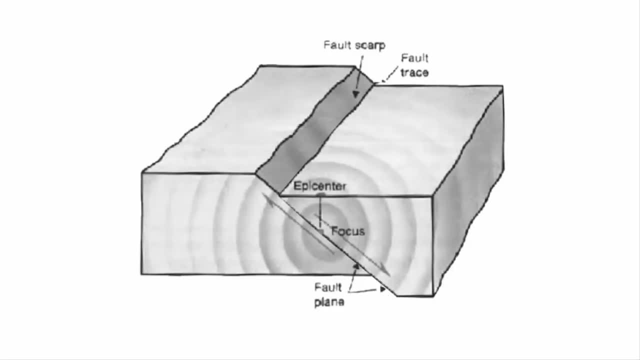 but at some point of time, their movements overcome the friction. As a result, they slide past one another. This causes the release of energy, and the energy waves travel in all directions. The point where the energy is released is called the focus of an earthquake, Or there is. 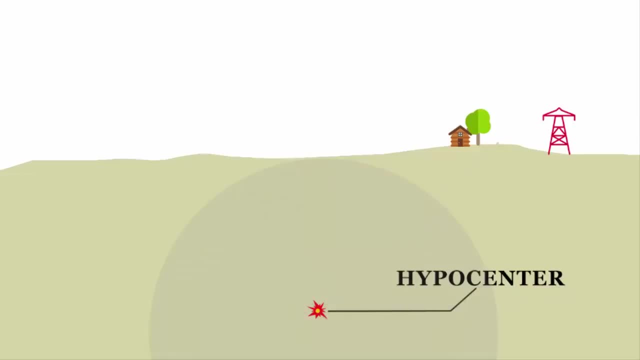 also a term given to it, called the hypocenter. The energy waves traveling in different direction reach the center of the earth. The energy waves travel in different directions, reaching the surface. The point on the surface nearest to the focus is called epicenter. This place is the first. 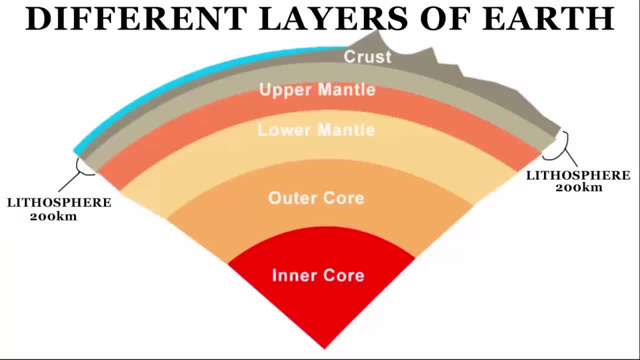 one to experience the waves. All natural earthquakes take place in the lithosphere. The lithosphere refers to the portion of depth up to 200 kilometer from the surface of the earth. An instrument called seismograph records the wave reaching the surface. The waves look something. 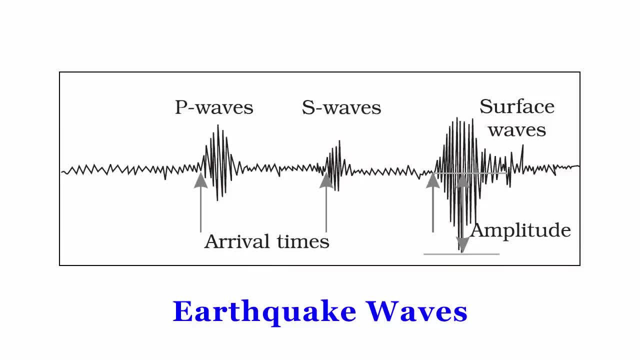 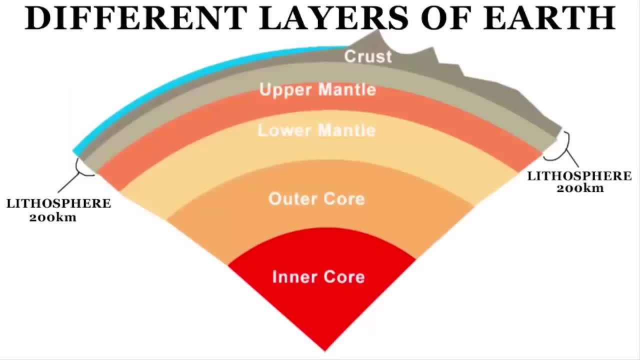 like this: The curve shows three distinct sections, each representing different types of wave patterns. We'll get back to this pattern in a moment. Earthquake waves are basically of two types: Body waves and surface waves. I need you to understand the term. body waves Sounds a little. 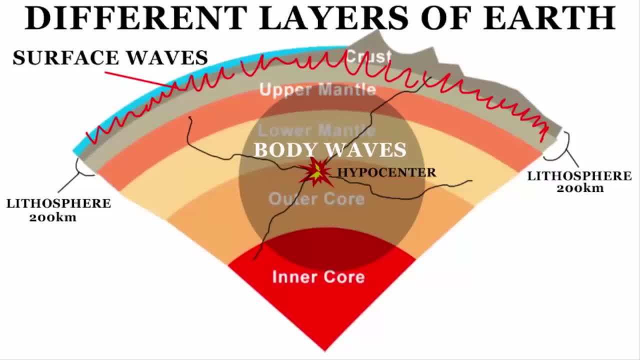 larger within the body right. So the body waves are generated due to the release of energy at the focus, that is the epicenter, and moves in all direction, traveling through the body of the earth. You know it travels internally, within the earth's surface, and moves the interior of the earth. 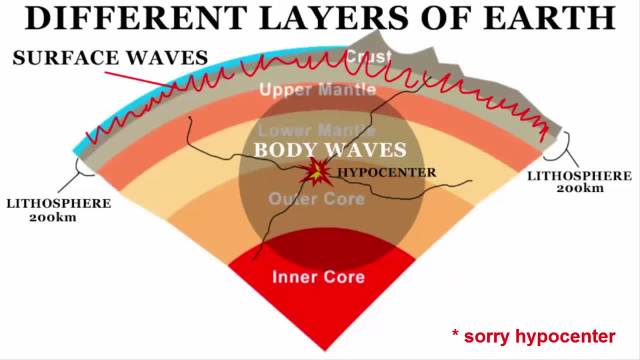 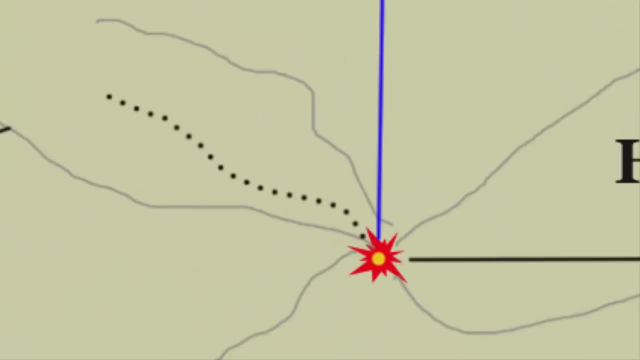 That's why it is referred to as body waves, because it is traveling through the body of the earth like a tremor. Now it is obvious that when these body waves move towards the surface, they will come in contact with the surface rocks and generate new set of waves. These are called surface 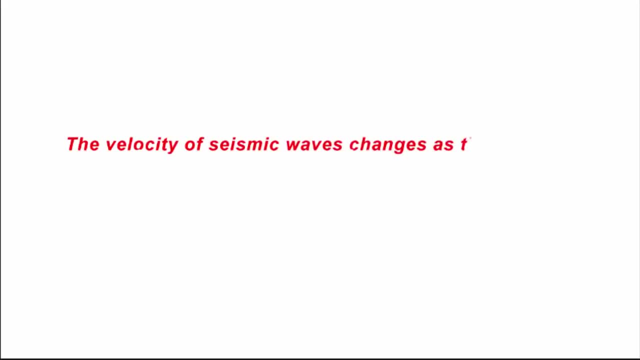 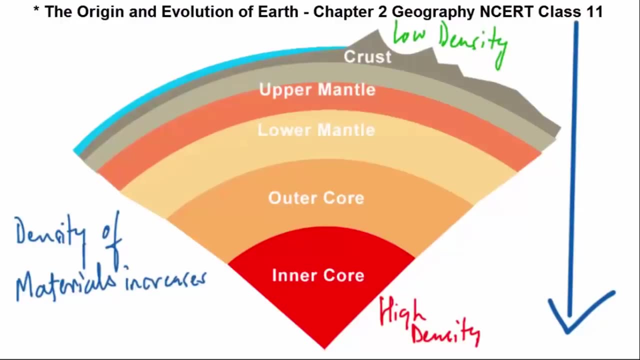 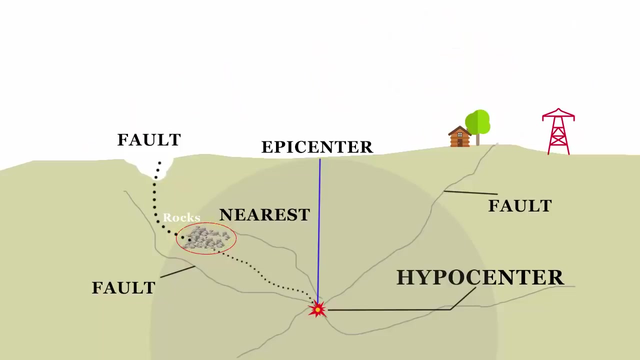 waves. Now, the velocity of waves changes as they travel through materials with different densities, And we know that the materials with higher density reside downwards. Therefore, the denser the material, the higher is the velocity. The direction also changes as they reflect or refract when coming across materials with different.